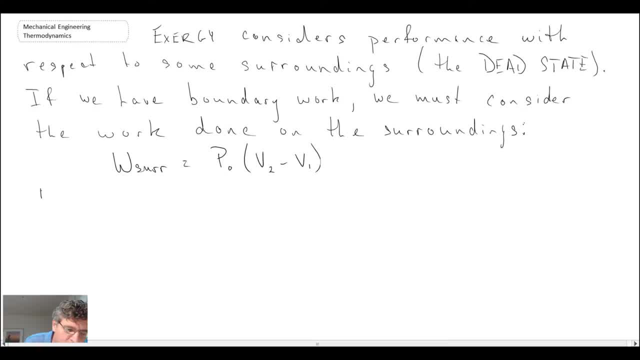 Exergy itself considers performance with respect to a dead state. So the amount of useful work that we get- and we'll denote that with a W subscript U- is equal to the work minus the work that we do on the surroundings and by substituting. 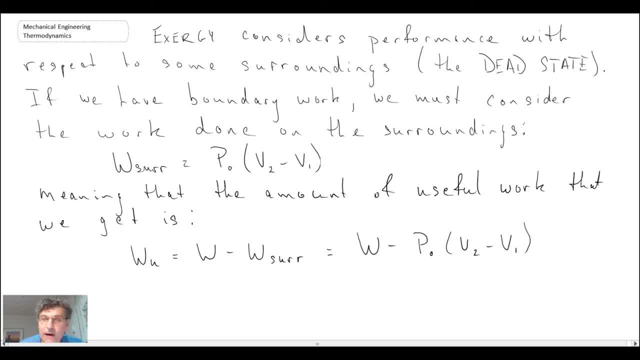 in the quantity that we said was for the work on the surroundings. the W here is the actual work being performed. So that is something that we have to be careful about. if we have a control volume, that is changing more. If we have a control volume, we need to take into account the fact that we may be doing 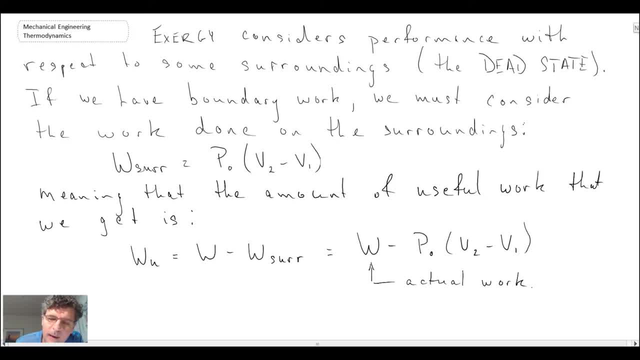 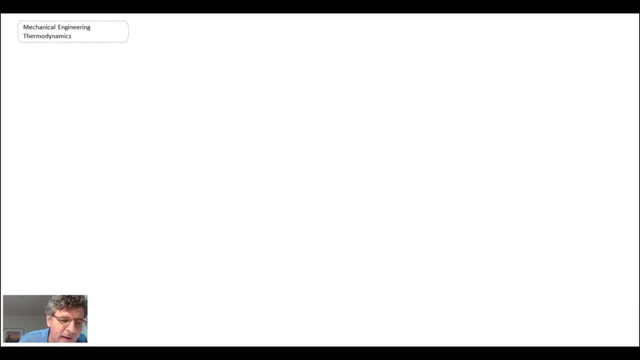 work on the surroundings, and there are two more terms- or I guess terms would be the best- that we should think about. One is reversible work, and we will talk about these. Reversible work is defined as being a, as being the maximum amount of useful work that can be produced. 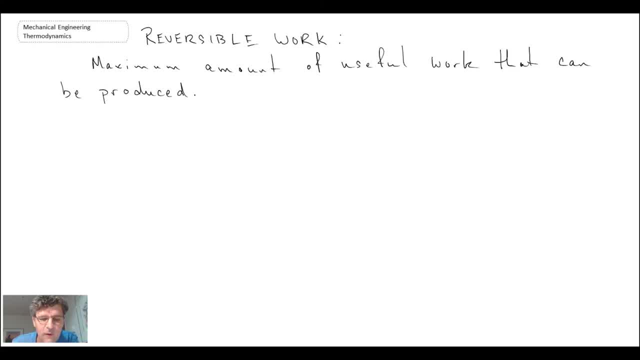 So that is what reversible work refers to and it makes sense. It would just be the maximum amount of work that you could produce if you had no irreversibilities in your system. So when we looked at the example of the Carnot heat engine a moment ago for the example problem, 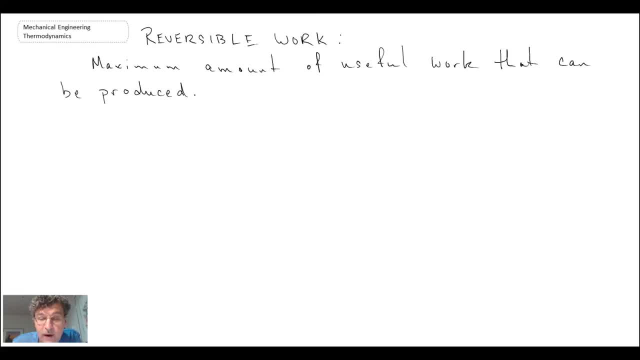 and we had the source at 1500 Kelvin. the amount of useful work coming out or reversible work was that from the Carnot efficiency. Another term that you'll hear discussed when we talk about exergy and exergy analysis is the term irreversibility. 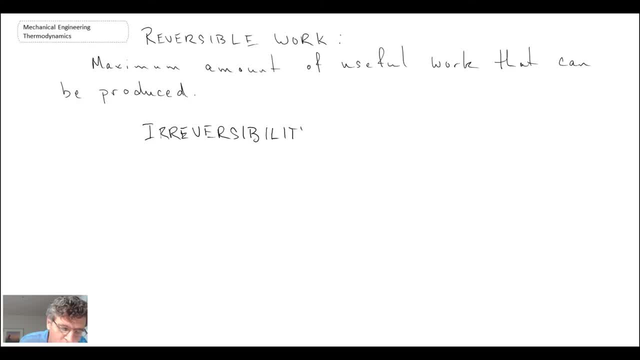 And what this is. it's basically exergy that is lost or destroyed through our process, So we want to minimize irreversibility as engineers. These are losses in our system, and irreversibility would be defined in two ways, depending on if we are looking at a system that is producing work or a system that we are doing work on. 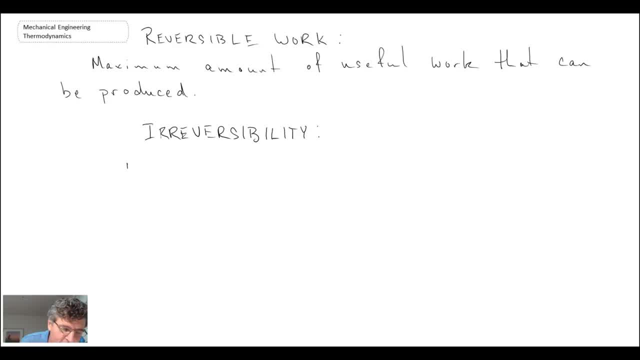 And so, taking a look at the first, where we have a system that produces work, irreversibility would be reversible work out minus useful work out. And if you have irreversibilities, what will happen is reversible work out is your ideal state. 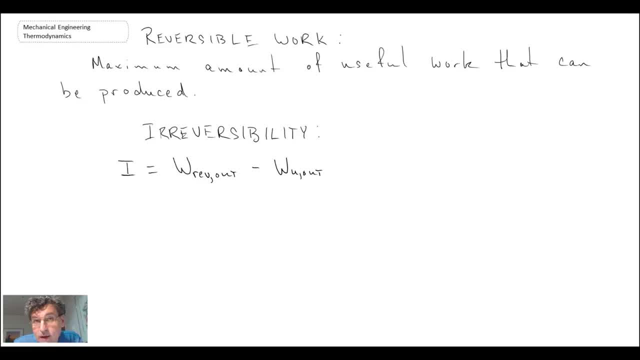 and it will always be larger than the actual or useful work that you get out of your system. Okay, consequently, irreversibility in this will always be a positive number, or you can have irreversibility expressed as useful work in minus, reversible work in and reversible work in on a device that you're doing work on, such as a pump or a.